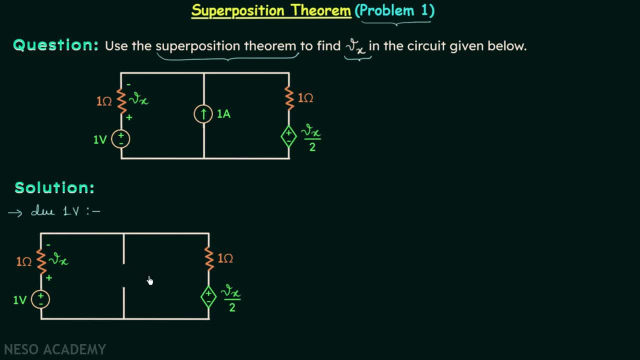 modification number one is we will open circuit this branch. and modification number two is we will rename this voltage. we will call it vx1 and because of this the voltage here will become vx1 by 2. now we want to find out vx1, we want to calculate this voltage, and for this we will. 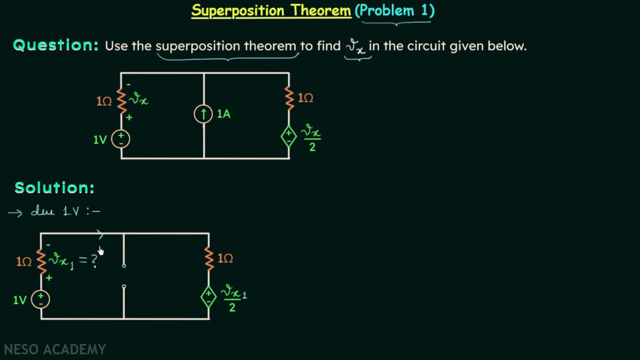 apply kvl in this loop. let's say the current is i1. so by applying the kvl we will have plus 1 plus 1, then we have minus vx1, minus vx1, then we have minus i1. multiplied to 1, that will be: 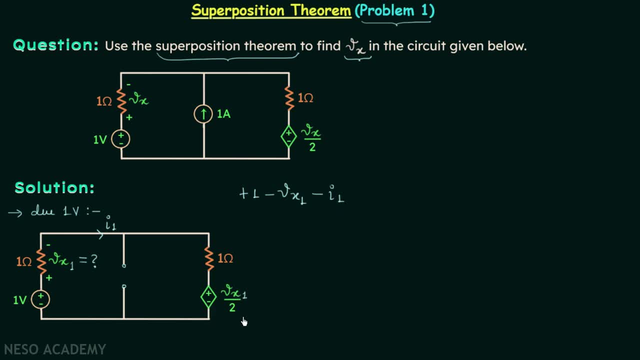 minus i1. after this, we will have minus vx1 divided by 2, minus vx1 divided by 2 equal to 0, and when you simplify this, you will have 3 over 2. vx1 plus i1 is equal to 1 and i will name this equation. 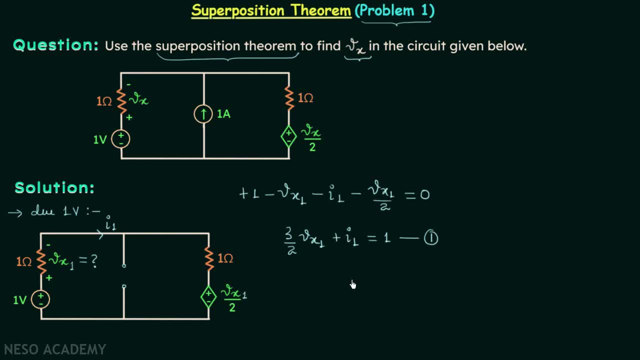 number 1. now, if we can write i1 in terms of vx1, we can easily have vx1 from this equation and to find out the relation between vx1 and i1, we will focus on this resistor. the voltage across this resistor is vx1 and the current through this. 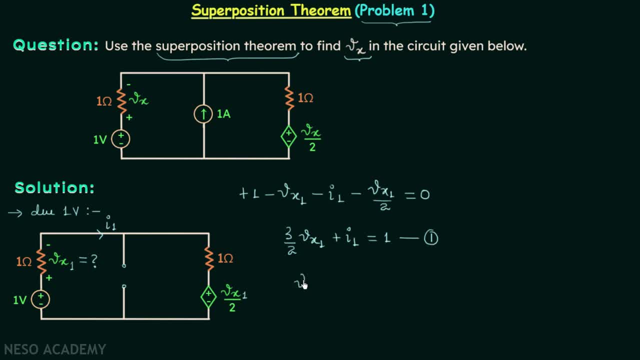 resistor is i1 and therefore we can say that vx1 is equal to i1 multiplied to the resistance, which is 1, so vx1 is equal to i1 and we can put i1 equal to vx1 in equation number 1. so from here we will. 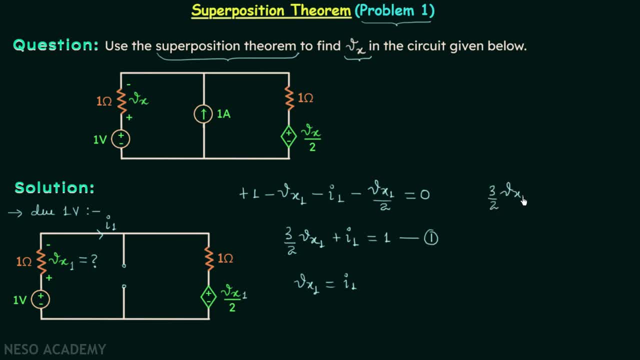 have 3 over 2 vx1 plus vx1 equal to 1, or we can say that we have 5 over 2 vx1 equal to 1. this implies the voltage vx1 is equal to 2 over 5 volts. so in this way we have obtained the voltage across this. 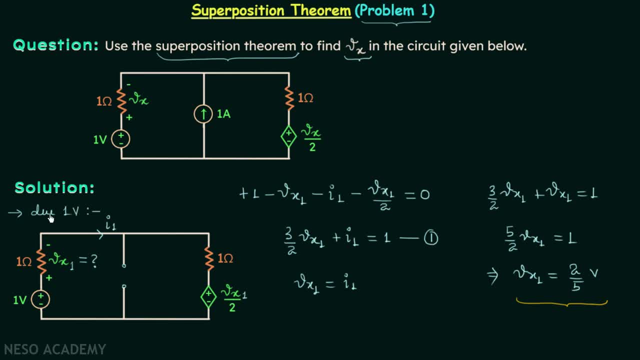 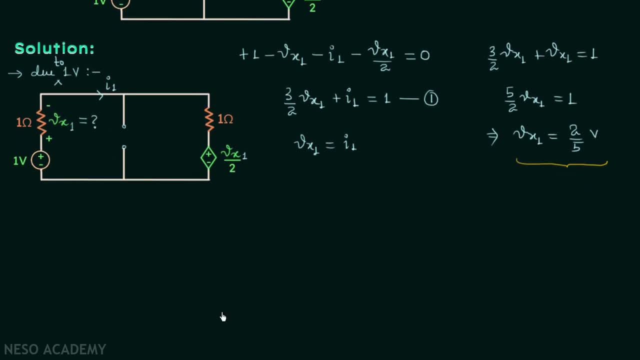 resistor due to 1 volt source. so we are done with our case number one. let us now move on to our case number two, in which we will find out the voltage across this resistor due to one ampere source, and for this purpose we will short circuit our independent voltage source. this is the first. 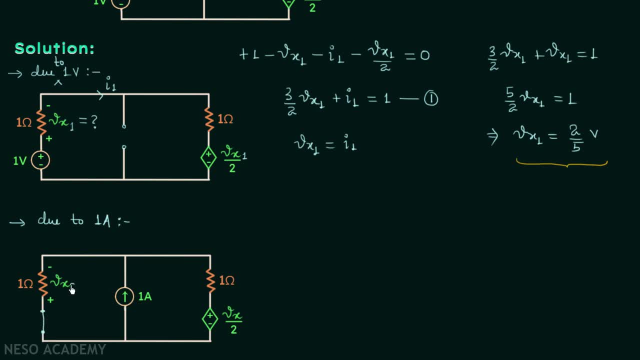 modification. and the second modification is renaming of this voltage and we will now focus on calculation of vx2. if we can have the current through this resistor, we can have vx2, and to find out the current through this resistor we will use nodal analysis. this is the reference. 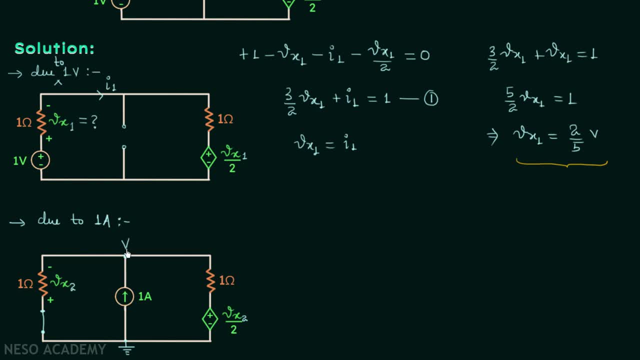 node, and this node here is our principal node, with voltage v. we know this voltage is the largest voltage and therefore currents will leave this node. let's say this is current i1, this is current i2 and this one here is current i3. the potential at this point is equal to zero volt and therefore 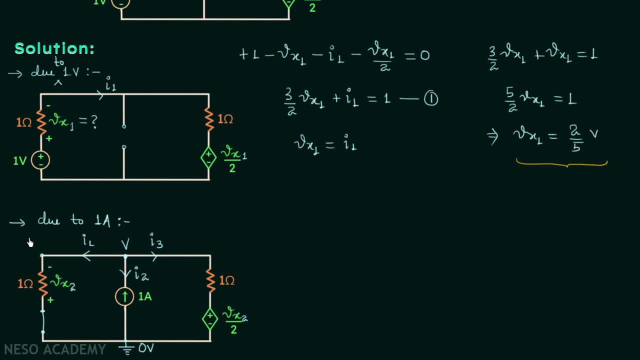 the potential at this point will be minus vx2, so the potential at this point will be minus vx2, minus vx2, and as there is no resistance in this wire, there will be no voltage drop and therefore v will be equal to minus vx2. v is equal to minus vx2 and the potential at this point will be plus. 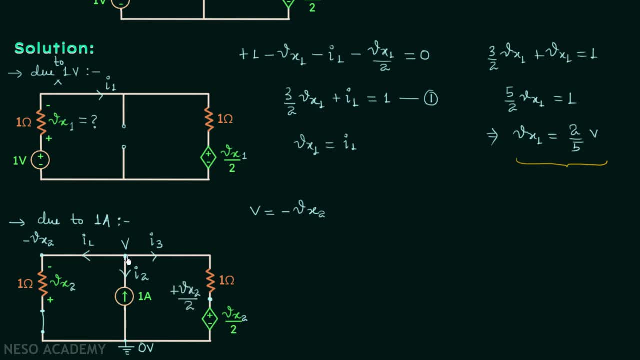 vx2 by 2.. now when you apply kcl at this node, you will have i1 plus i2 plus i3, equal to zero. current i1 is equal to v minus 0 divided by 1, so we have v. current i2 is simply equal to. 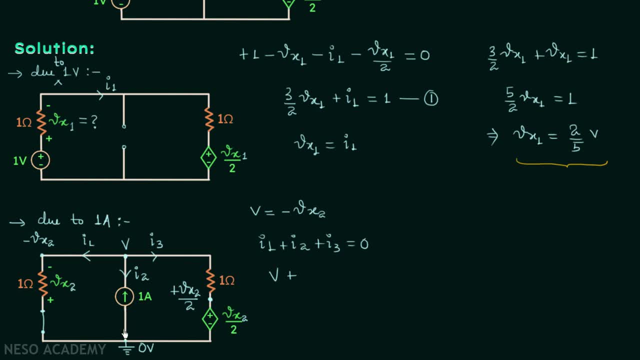 minus 1 ampere, because this is the current in this branch, but in opposite direction. so we have minus 1 current i3. it is equal to v minus vx2 by 2 divided by 1. so we have v minus vx2 divided by 2.